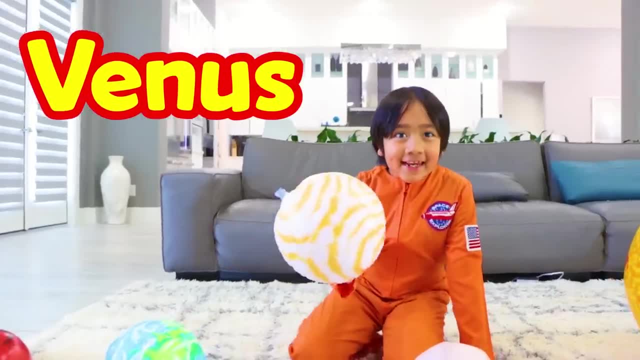 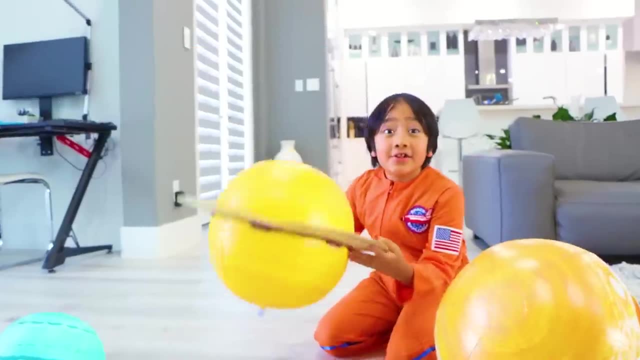 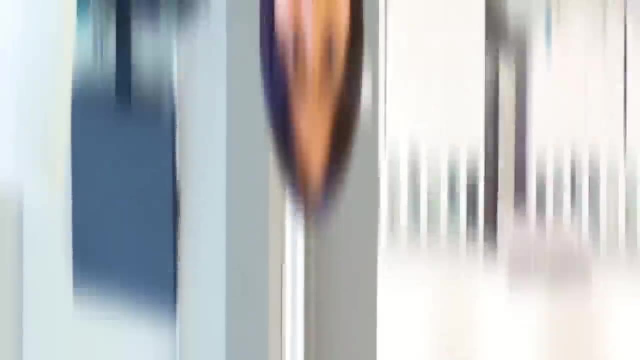 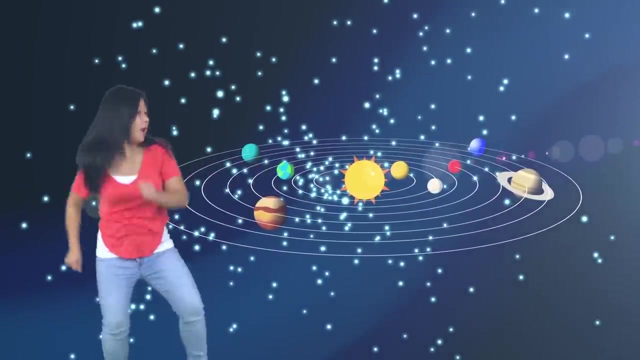 My for Mercury, Very for Venus, Excellent for Earth, Mother for Mars, Just for Jupiter. Served for Saturn, Us for Uranus And noodles for Neptune. Here's also a very fun song to help learn the planets. This is the planet song. 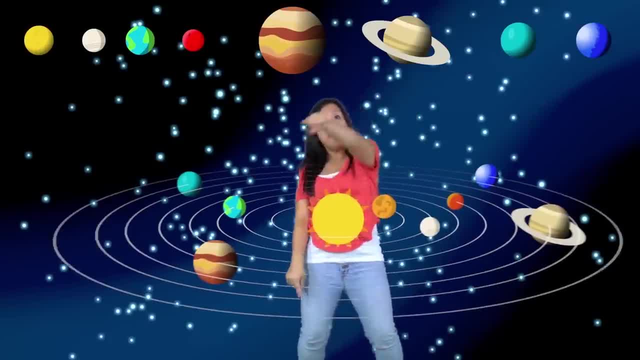 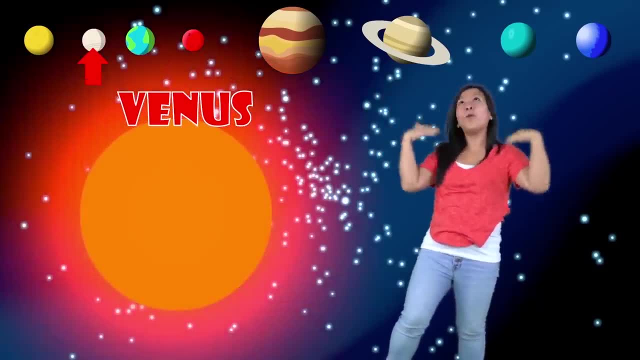 If you know the order, sing along. Planets revolve around the sun. Mercury is number one, Venus is number two. It's too hot for me and you. Earth is the place to be. It's planet number three. Now let's learn some more. 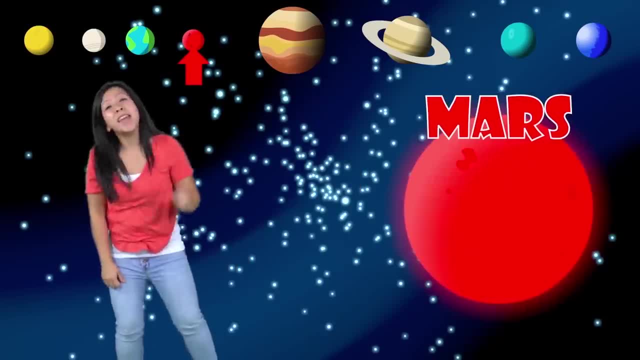 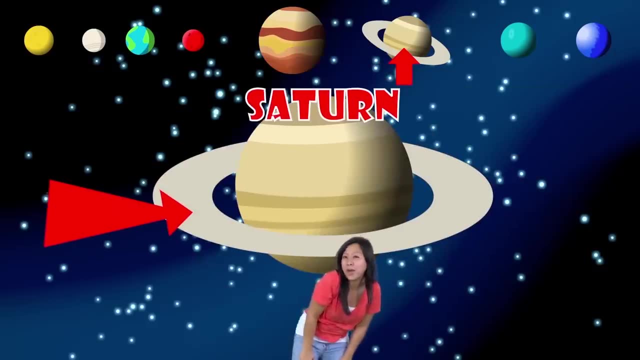 Mars is red and it's number four. Jupiter is number five And it's known for its giant size. Saturn is the one with rings. It's number six in the order of things. Seven is the planet with ice: It's Uranus, and it's been on Earth for a long time. 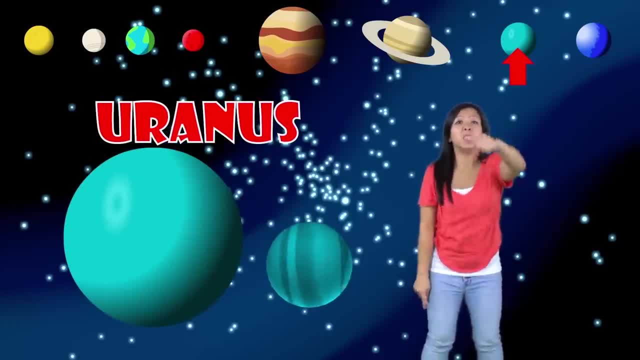 And it's known for its giant size. Saturn is the one with rings. It's number six in the order of things And it's known for its giant size. Number eight's called Neptune. It's the last one and it's blue. 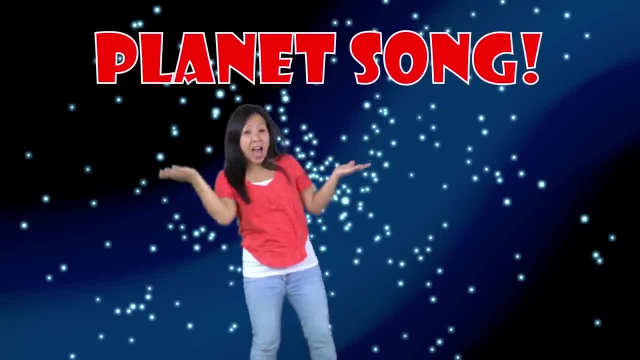 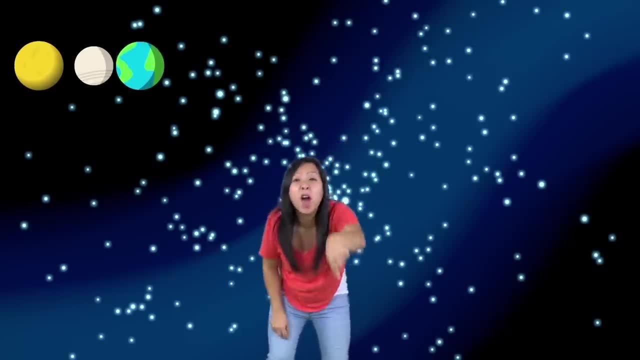 This is the planet song. Now you know the order. sing along: Mercury, Venus, Earth, Mars, Jupiter, Saturn, Uranus and Neptune. Mercury, Venus, Earth, Mars, Jupiter, Saturn, Uranus and Neptune. 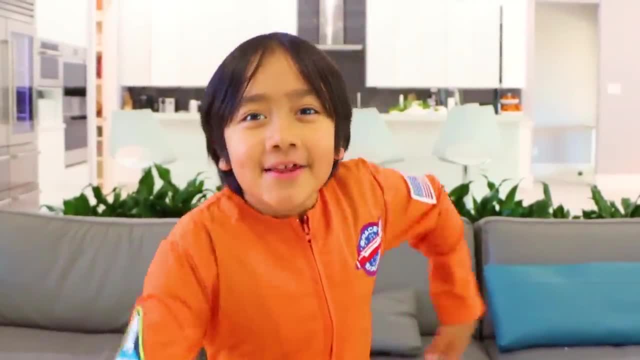 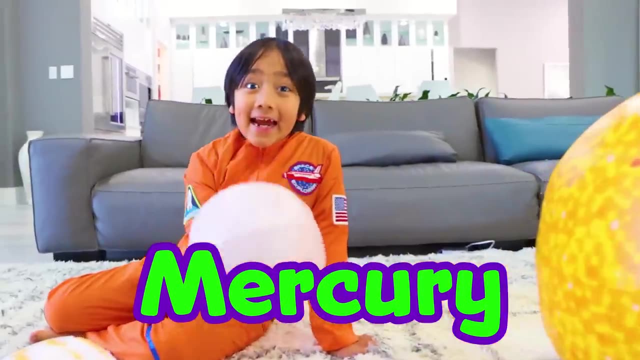 Ready to learn some fun facts about each planet with me, Let's do it. The first planet that is also the closest to the Sun is Mercury. The first planet that is also the closest to the Sun is Mercury, And it's also the smallest planet. 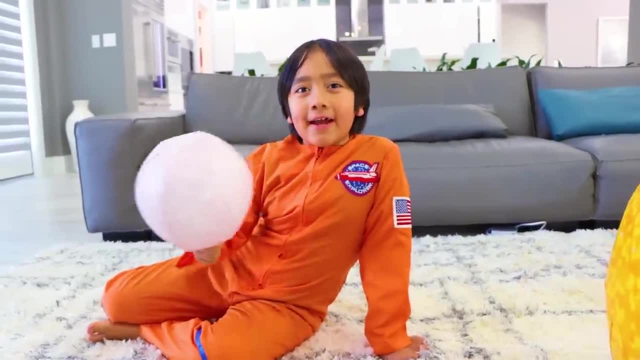 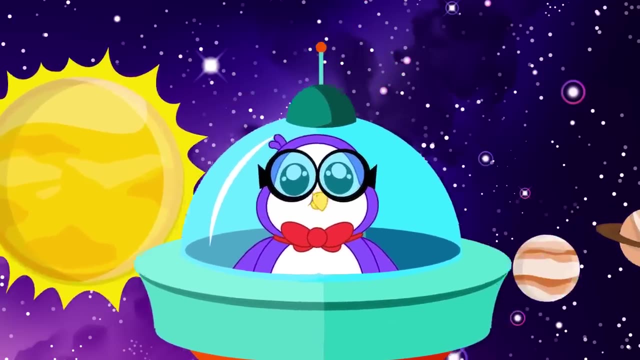 I'll have Peck tell you more about Mercury. I'll have Peck tell you more about Mercury. Thanks, Ryan. I'm so excited to share some facts about the planets. I'm so excited to share some facts about the planets. Let's start with Mercury. 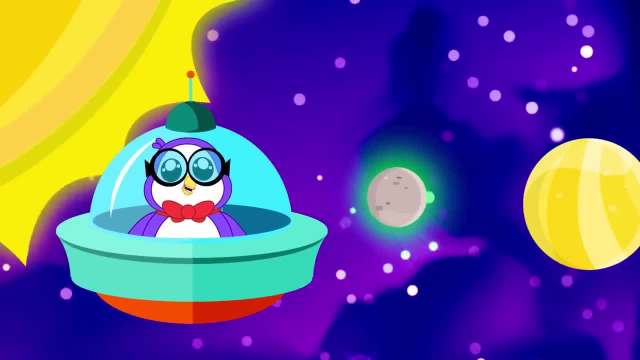 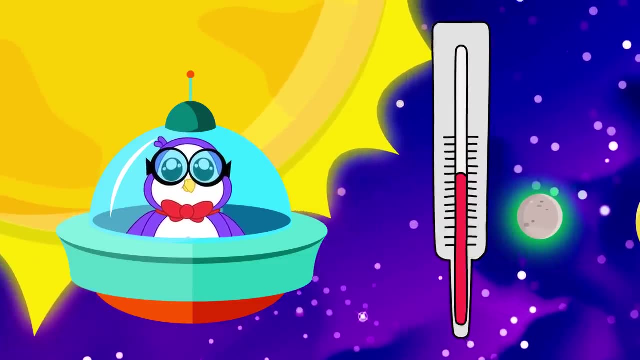 Mercury is the smallest planet. It does not have any moons or rings. It does not have any moons or rings. Even though Mercury is the closest planet to the Sun, it's only the second hottest planet. It's only the second hottest planet. 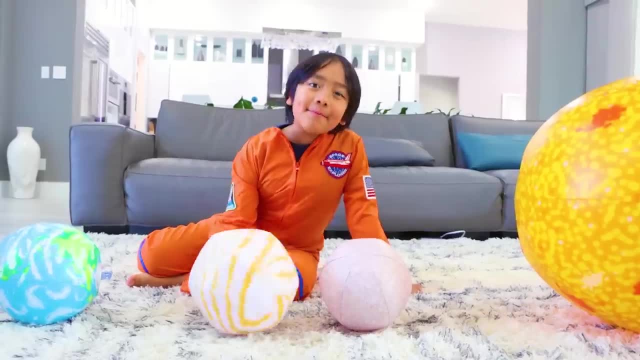 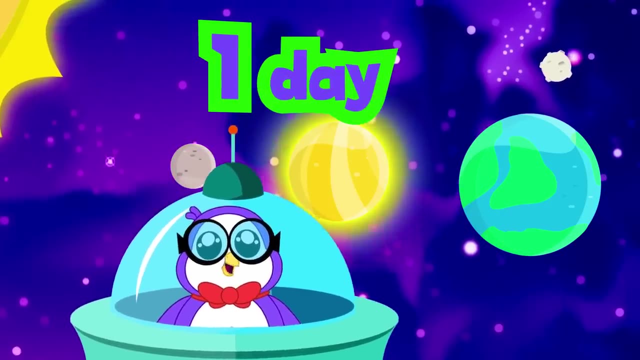 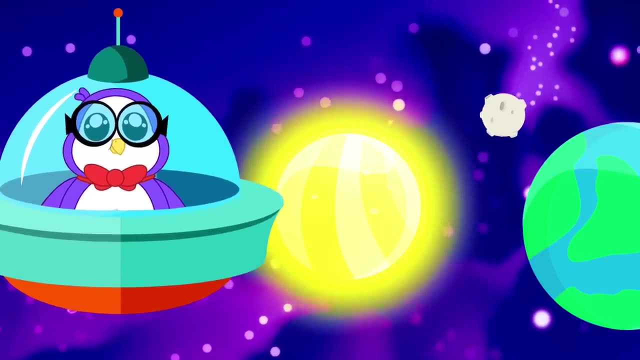 Mercury takes only 88 Earth days. The second planet is Venus. Peck, tell us more about Venus. Did you know one day on Venus lasts 243 Earth days. Venus is the second brightest object in the night sky. Only the moon is brighter. 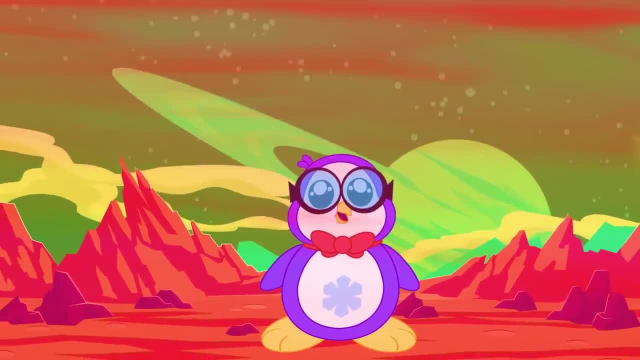 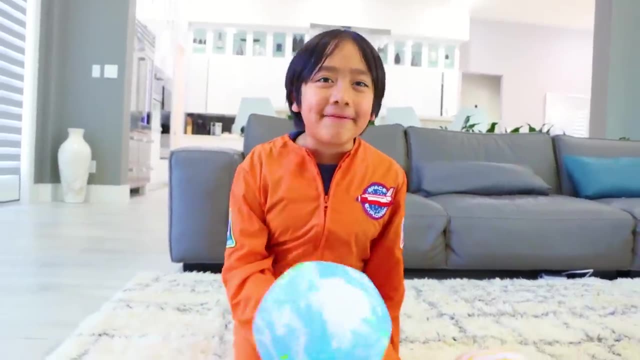 Because of its harsh atmosphere, Venus is the hottest planet in the solar system. The third planet from the sun is Earth. It's also my favorite because we live here. Okay, Peck, It's your turn to tell us some fun facts about Earth. 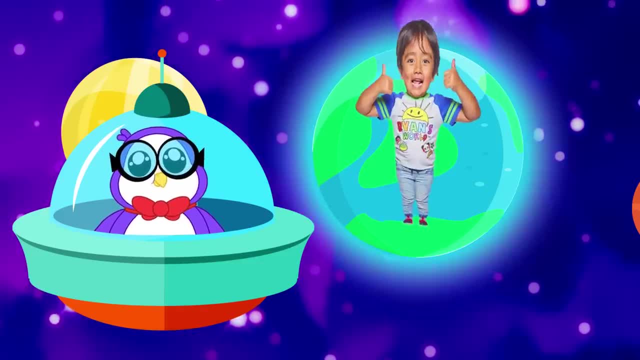 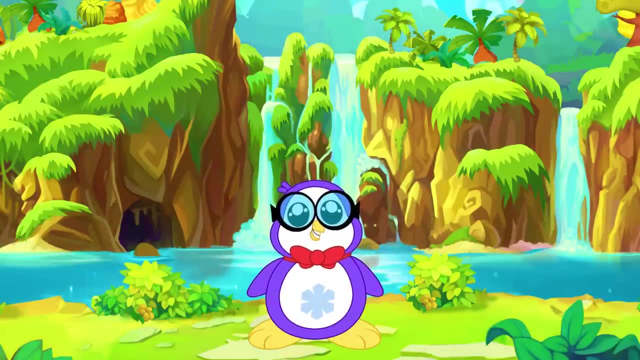 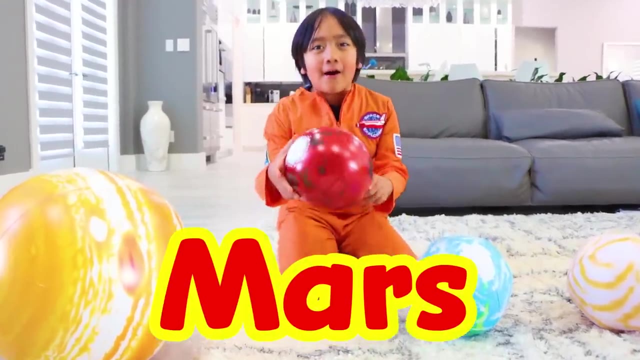 Earth is the only known planet to support life. 71% of the Earth's surface is covered in water, Although 3% is freshwater and 2% is frozen in ice sheets and icebergs. Next up planet is Mars. It's also sometimes called the red planet. 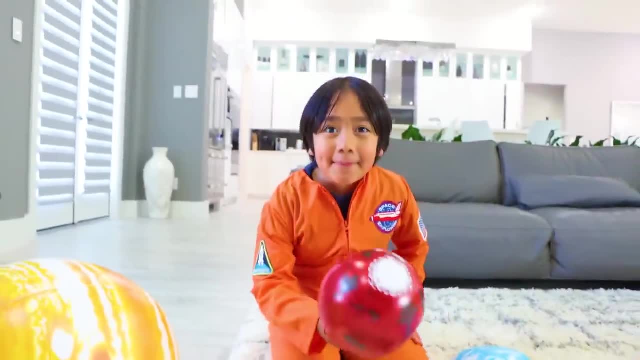 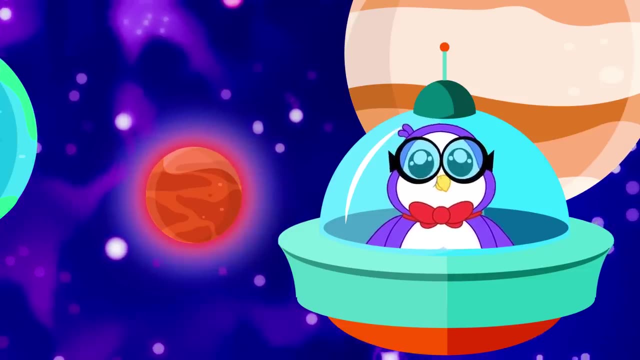 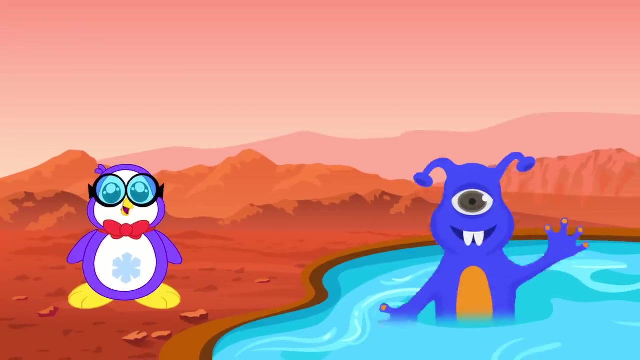 because it looks warm. It's red from Earth. Okay, Peck, Now tell us some fun facts. Mars is known as the red planet due to its reddish appearance. Unlike other planets, there are signs of liquid water on Mars, which means maybe it could one day support life. 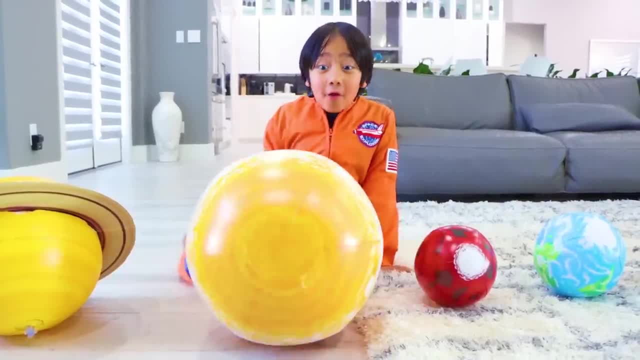 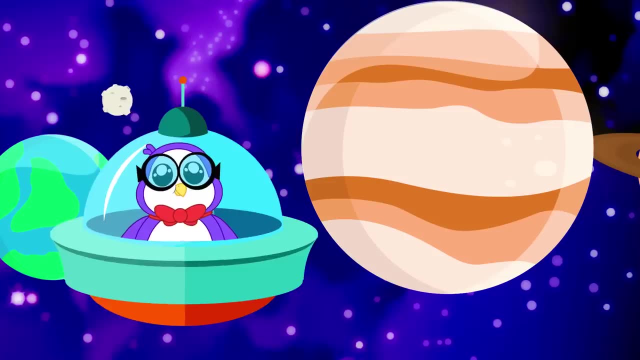 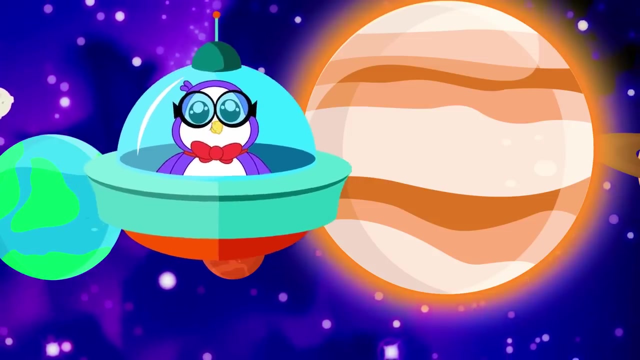 The fifth planet from the sun is Jupiter. It's also the largest planet in our solar system. Okay, Peck, Can you tell us some fun facts about Jupiter? Jupiter is the largest planet in the solar system, Whoa. It's primarily made up of gas and is therefore known as the gas giant. 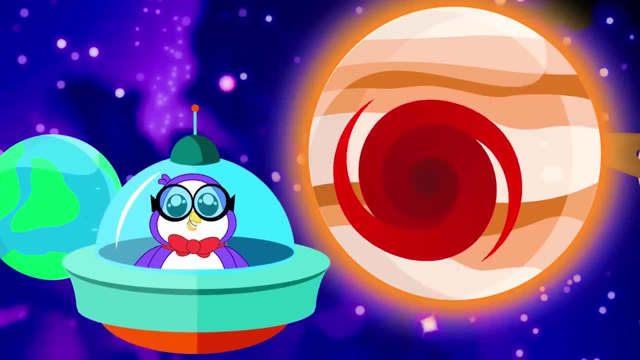 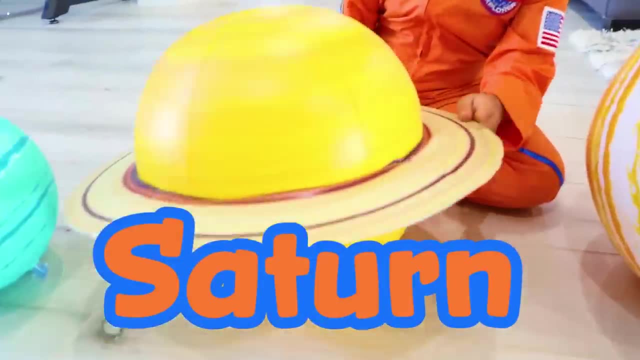 The Great Red Spot is a huge storm on Jupiter that is the size of three Earths. This is the sixth planet from the sun, It's Saturn. And you see these rings? They're actually made out of millions of ice chunks. Okay, fun facts with Peck. 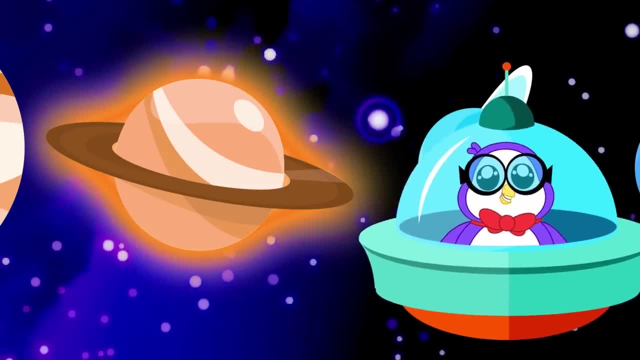 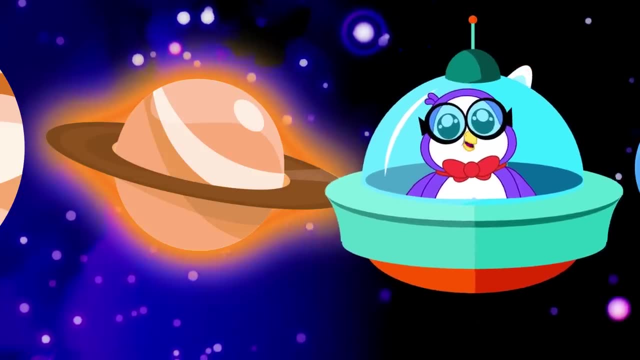 Whee. Saturn is another gas giant. It's the largest planet in the solar system. It has the most extensive rings that are made up of ice chunks and dust. Saturn has 82 moons. The seventh planet from the sun is Uranus. 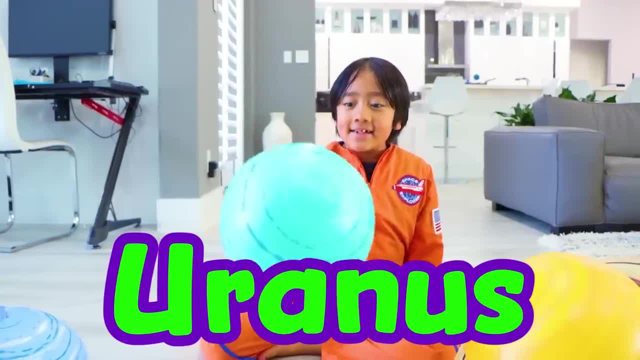 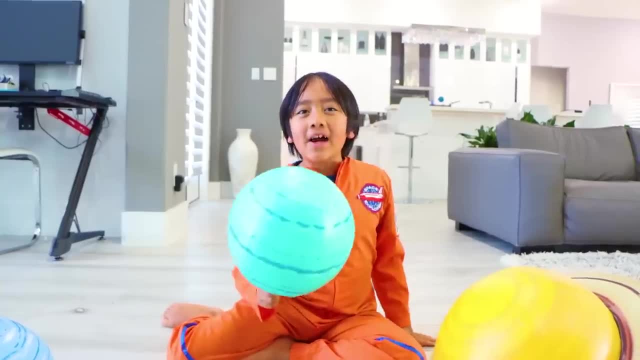 And it appears to spin on its side. And Peck will tell you some more fun facts about Uranus. Uranus is not visible to the naked eye and is the first planet discovered by the use of a telescope. It is referred to as an ice giant planet. 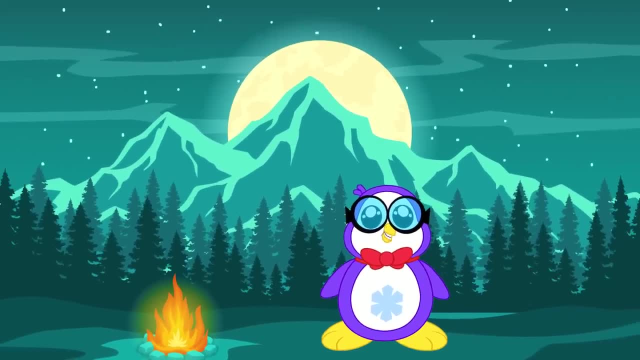 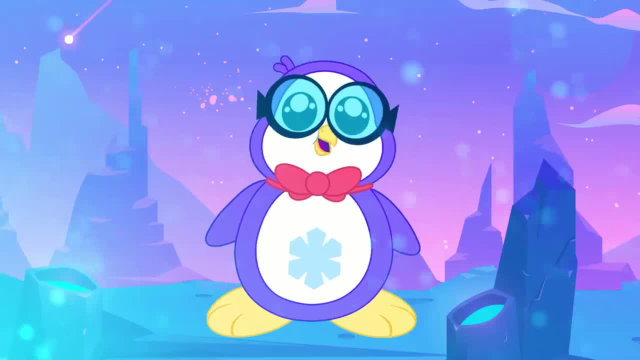 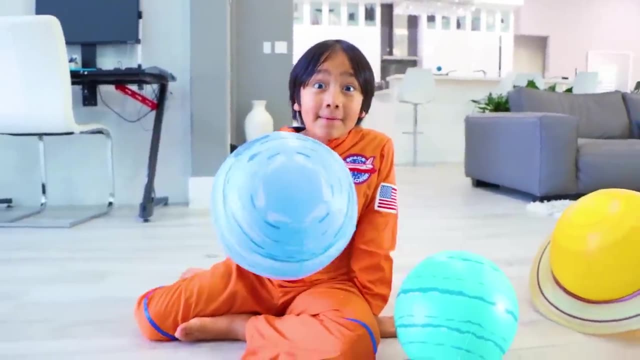 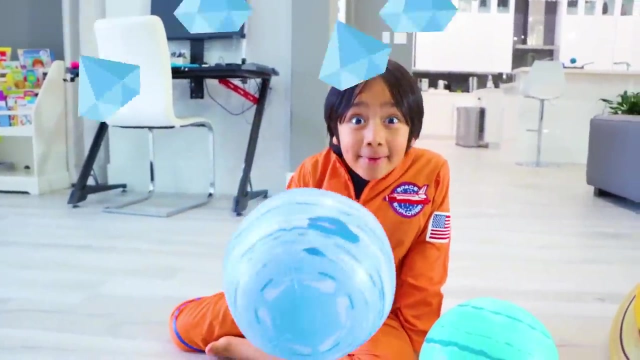 It's a giant planet. It's a giant planet. It's a giant planet. Although it's not frozen, the atmosphere is filled with ice crystals. The eighth planet from the sun is Neptune, And since it's so far away from the sun, it is super dark and cold here and it rains. 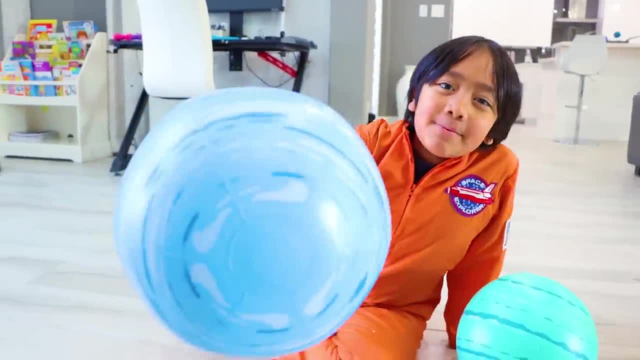 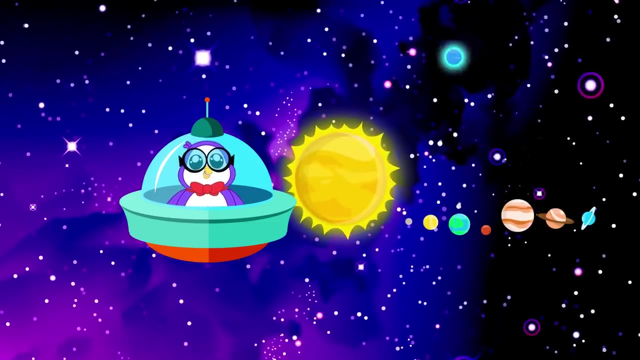 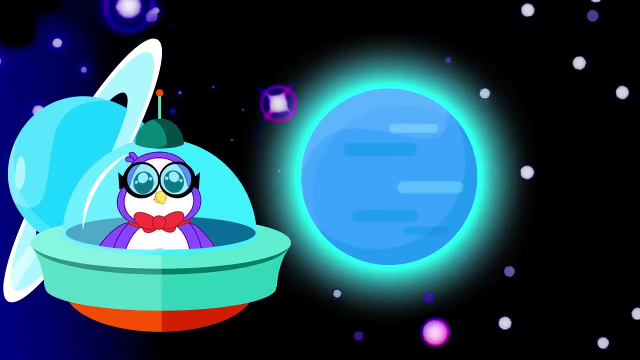 diamonds, Cha-ching. Okay and Peck will tell you some more fun facts about Neptune. Whee, Neptune is the most distant planet from the sun. Son a year on Neptune lasts longer than 165 years on Earth. All the methane in Neptune's atmosphere gives it its blue color. 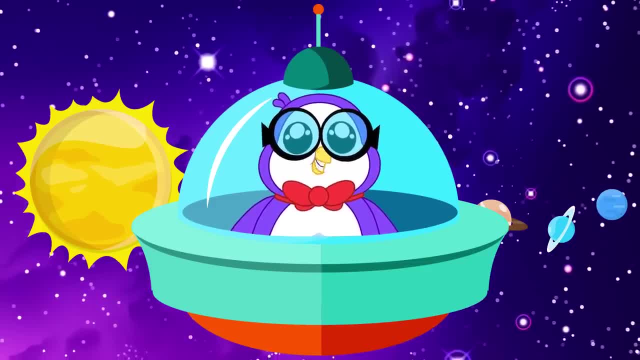 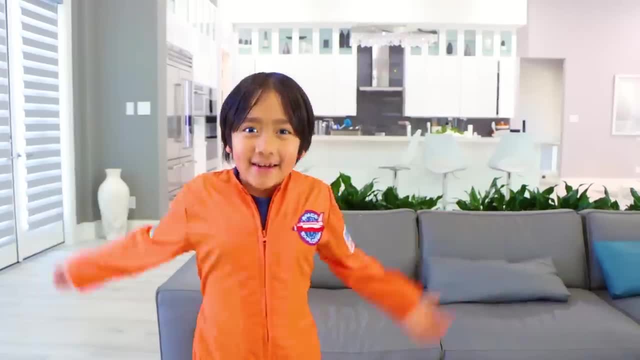 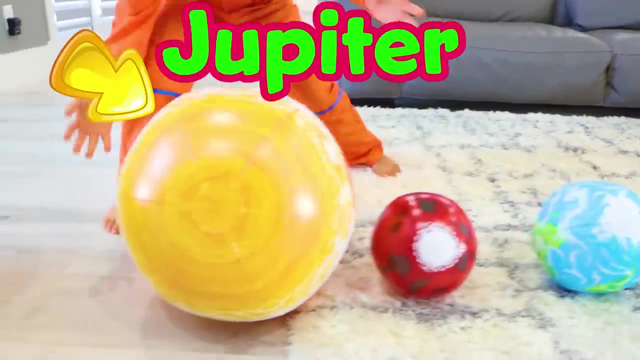 Wow, learning about the planets was fun, Ryan. See you later. Recap time. How many planets are there in the solar system? There are eight. It is Mercury, Venus, Earth, Mars, Jupiter, Saturn, Uranus and Neptune. 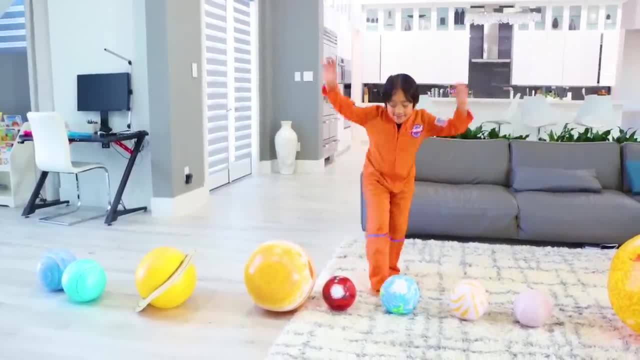 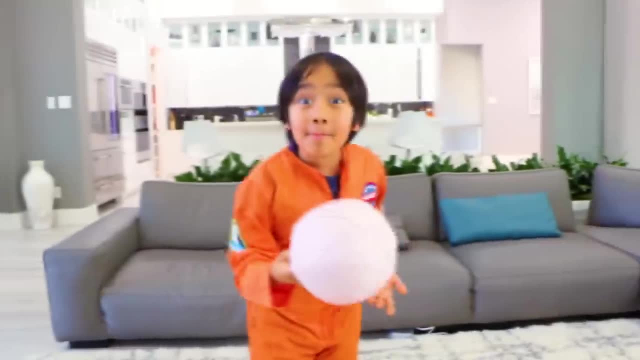 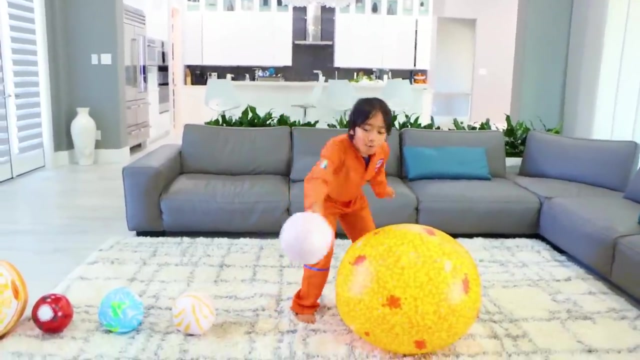 All of these planets orbit or go around the sun like this: That's one year, 365 days. Some planets orbit the sun super fast, like Mercury. It only takes 88 days, since it's the closest. Whee, Oh, You're there. 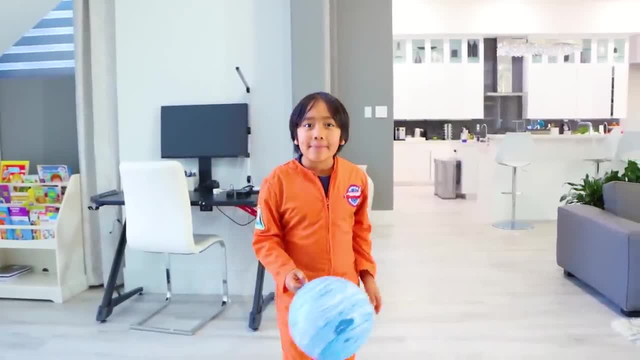 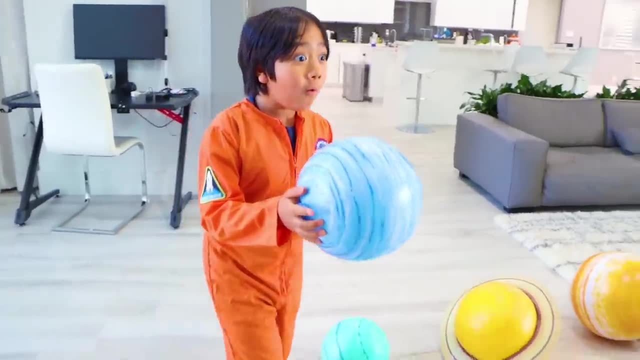 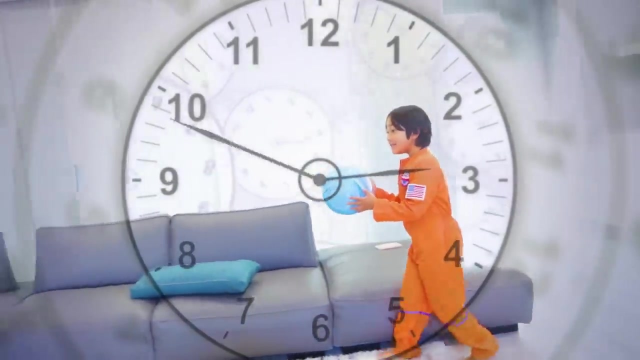 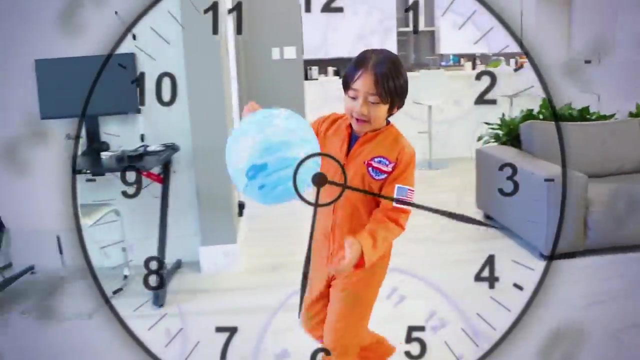 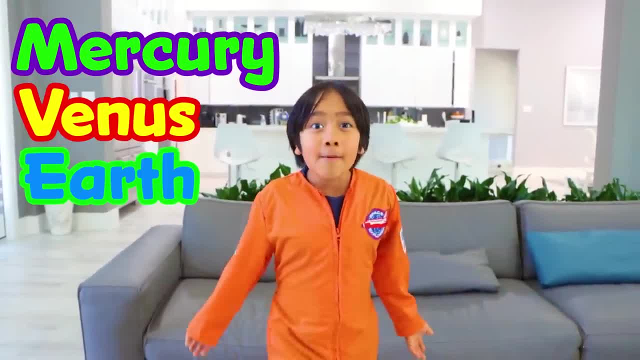 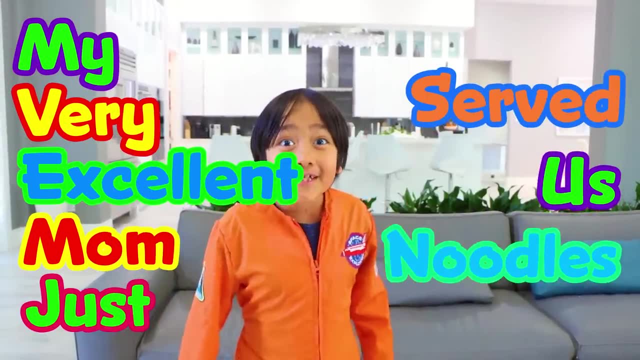 Is it the order? again? It's Mercury, Venus, Earth, Mars, Jupiter, Saturn, Uranus and Neptune. My very excellent mom just served us noodles. Okay, guys, thank you for learning all about the planets with me. Remember: always stay happy and Ryan. 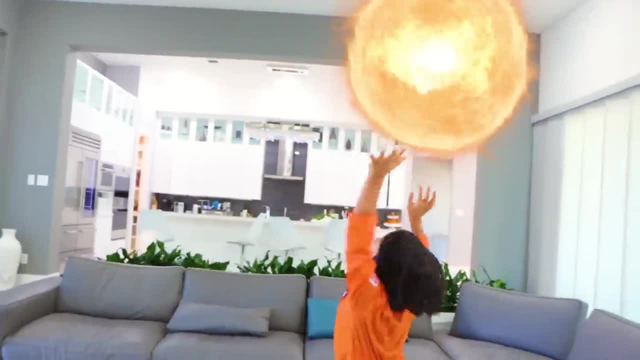